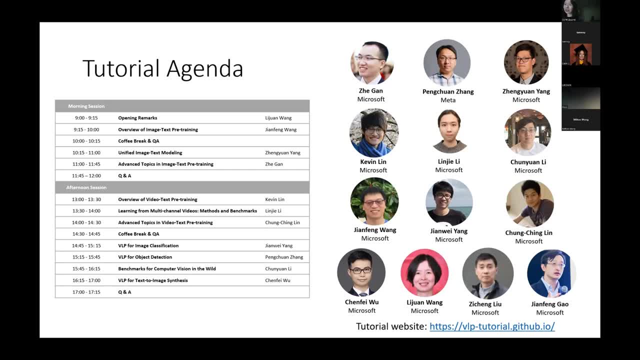 various topics related to recent advances of vision and language pre-training. The VLP pre-training is divided into four pillars, So such as image text pre-training, video text pre-training, VLP for vision and vision language pre-training. The VLP pre-training is divided into four pillars, So such as image text pre-training. 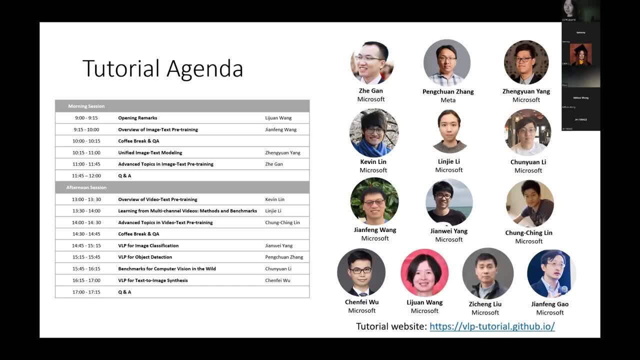 video text pre-training and vision language pre-training. So in today's morning session we will talk about image text pre-training And in afternoon session we will cover both the video text pre-training and the VLP for vision. So we want to talk about the VLP in today's tutorial. 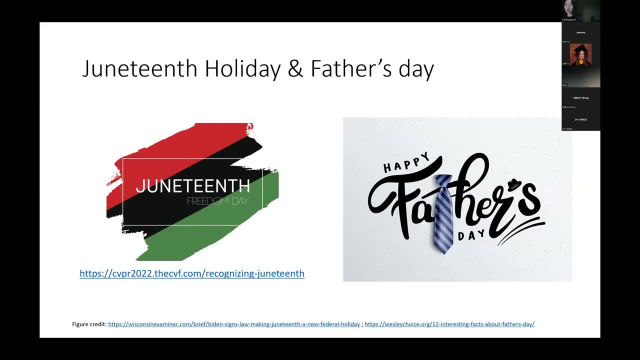 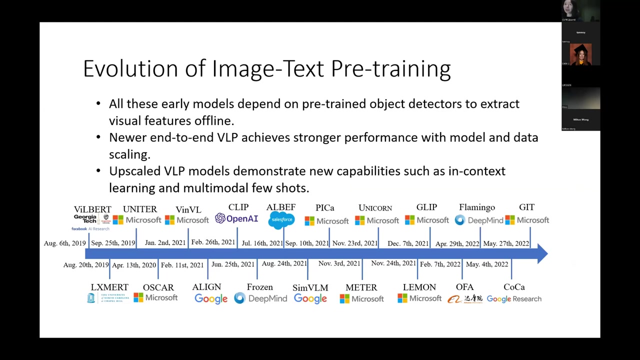 And also today in New Orleans. so we are celebrating a federated holiday for Juneteenth, And today is also Father's Day, So we wish all the fathers at the CVPR a happy Father's Day. At first, we will briefly review the evolution of image text pre-training. 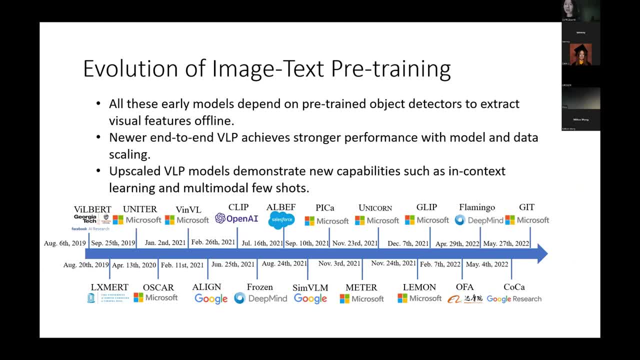 So the journey of the image text pre-training is very short. So the journey of the image text pre-training is very short. So the journey of the image text pre-training starts in the summer of 2019, with models like VL, BERT, LexMert and UNITR leading the way. 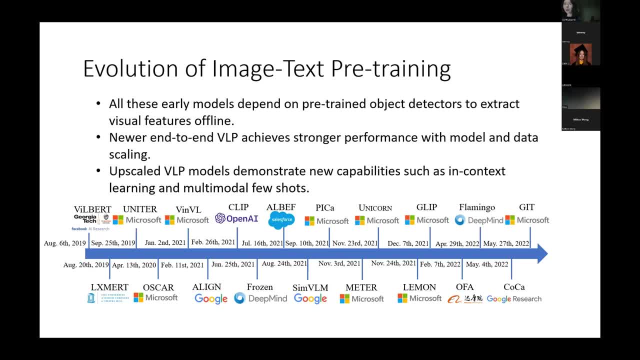 Follow-up like OSCA and VimVL, with improved visual features and object text. Newer end-to-end VLP models such as SimVLM, METR, Flamingo, COCA and GIT, achieves stronger performance with much larger model and also with large amount of image text. pre-training data. 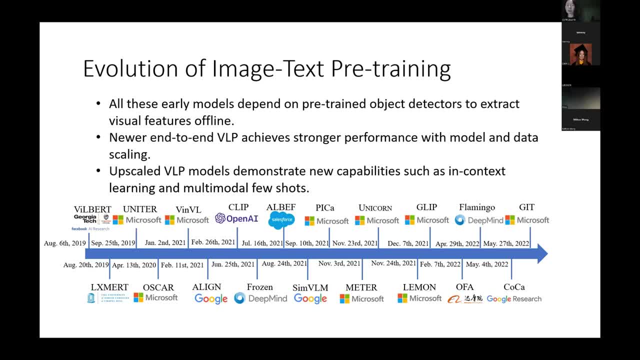 In the meanwhile, these upscaled VLP models is beginning to demonstrate new capabilities, such as in-context learning and multi-model view shots. The representative models include Frozen Flamingo and COCA and PICA. The representative models include Frozen Flamingo and COCA and PICA. 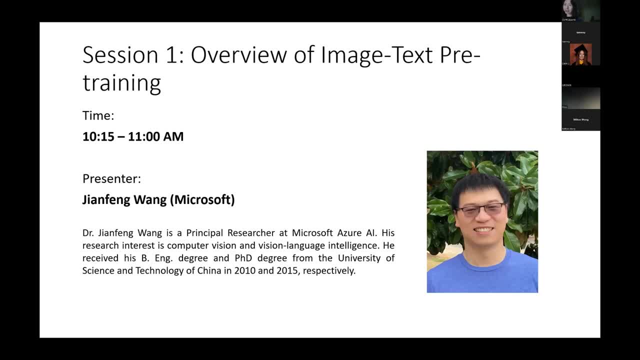 So the journey of the image text pre-training starts in the summer of 2019, with models like VL, BERT, LexMert and UNITR leading the way, Follow-up like OSCA and VimVL, with improved visual features and object text pre-training. 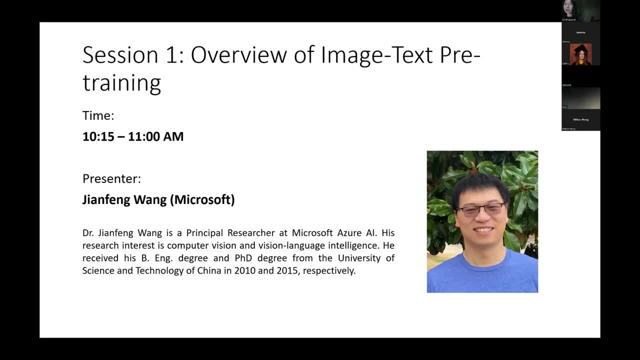 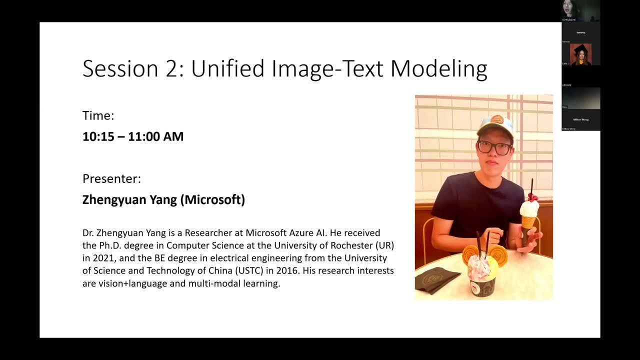 As a result of this, the team has also made improvements to their image text pre-training and are doing work on it towards the end of 2021.. So in today's morning session we were talking about the image text pre-training part. After Jianfeng's talk, we will have a short coffee break. 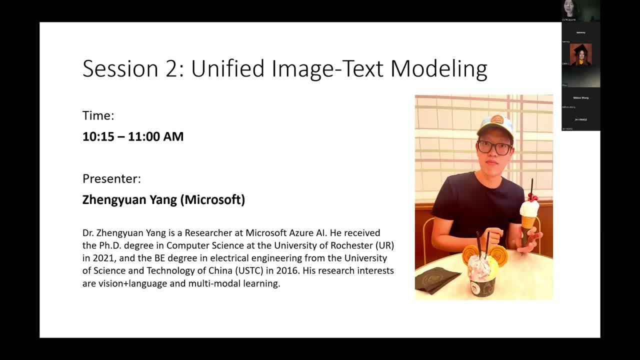 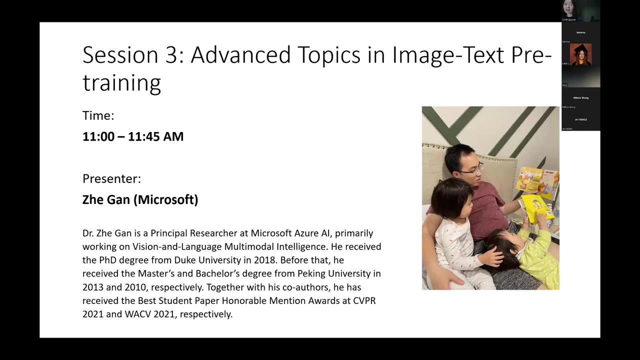 And after coffee break, Zhenyuan will present on Unified Image Text Modeling. Zhenyuan is also a researcher at Microsoft Azure AI. His research interests are vision language and multimodal learning. Followed Zhenyuan's talk, Zhe Gan will present on Advanced Topics in Image Text Pre-training. 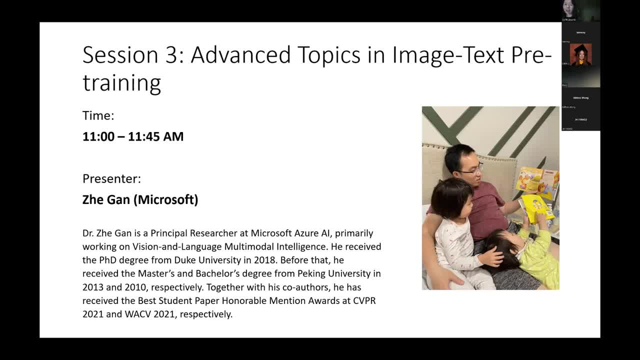 Zhe is a principal researcher at Microsoft Azure AI, primarily working on vision and language multimodal intelligence. He is also the recipient of the Master's Degree in Mathematics at the University of New York. He is also the recipient of the Master's Degree in Mathematics at the University of New York. 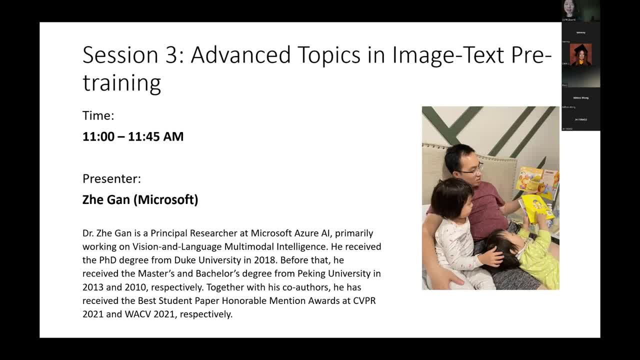 Liao has won three divisions of the Best Student Paper, honorable mentions awards at the CDPR 2021 and the WAC 2021.. After Zhenllen's session, we will have a Q&A session for all the morning talks and followed is the lunch break. 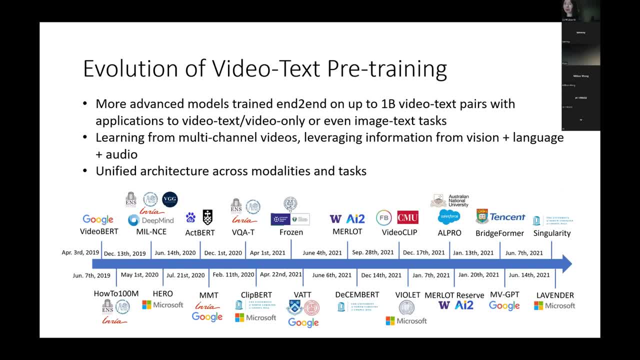 In the afternoon we will talk about video text pre-training part. There has been a lot of discussion on teaching math tonight. there has been significant advances in video pre-training. video text pre-training Started from the early work, like Video Bird from Google. 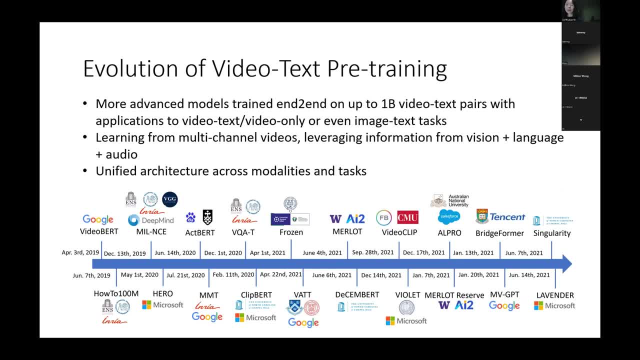 and also How to 100 Million, from INRIA to the most recent models like Mallotte Reserve, like MVGPT, Singularity and Lavenda, We see that more advanced models, trained in end-to-end manner on up to 1 billion video taxpayers can be applied to different applications. 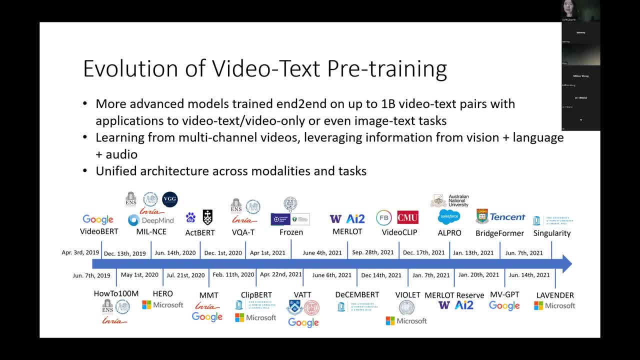 including to video text, video only or even image text task. We also see that the trend is like the future: video text: pre-training models can learn from multi-channel video. leveraging information from video. video text pre-training models can learn from multi-channel video. 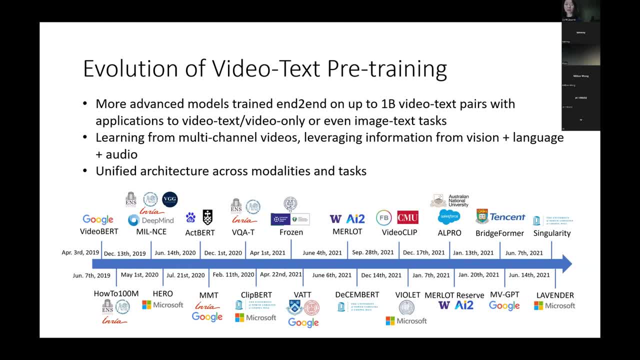 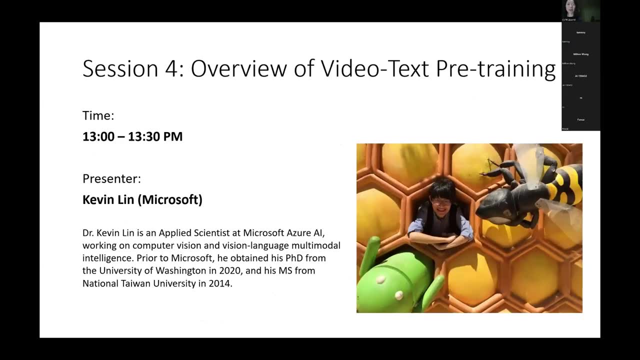 leveraging information from vision plus language plus audio. We believe in the unified architecture across modalities and the tasks is the future of video text pre-training. The afternoon session will start at 1 pm, So the first session will be presented by Kevin Lin. 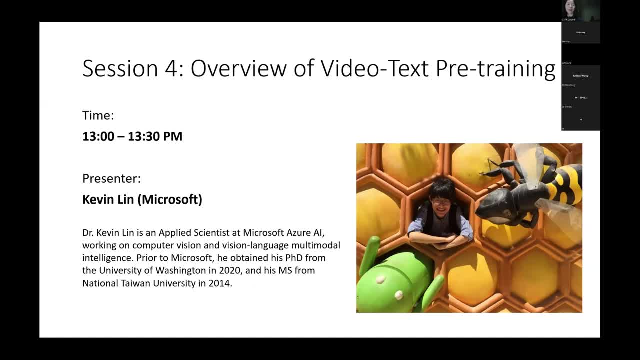 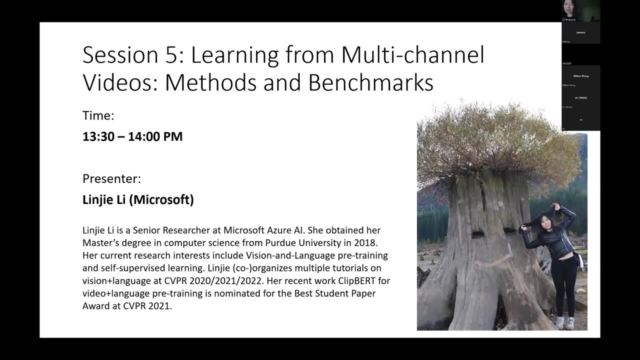 on overview of video text pre-training. Kevin is an applied scientist at Microsoft Azure AI, working on computer vision and vision language multimodal intelligence. After that, Linjie Li will present learning from multi-channel videos covering both methods and benchmarks. Linjie is a senior researcher at Microsoft Azure AI. 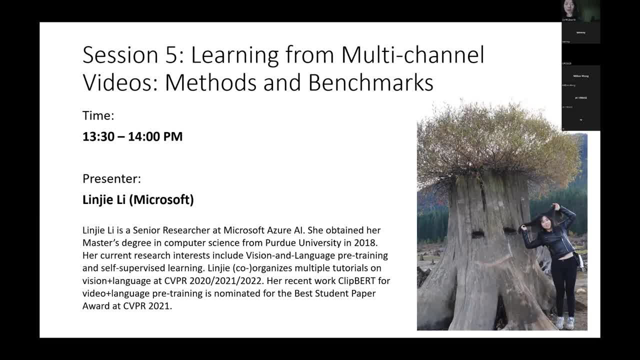 She co-organizes multiple tutorials on vision and language at CDPR 2020,, 2021, and 2022,. this year, Her recent work Cliff Burt for video language pre-training is nominated for the best student paper award at CDPR 2021.. 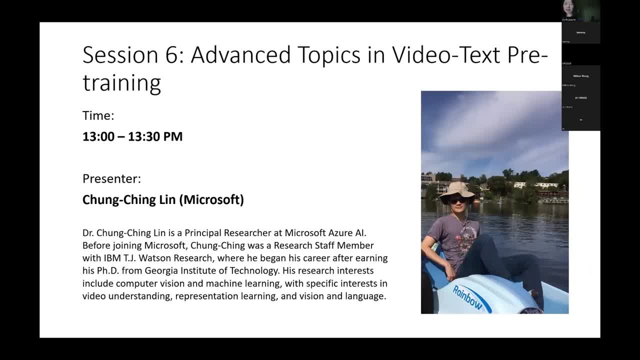 After that, Chongqing Lin will present advanced topics in video text pre-training. Chongqing is a principal researcher at Microsoft Azure AI. His research interests include computer vision and machine learning, with a specific interest in video understanding, representation learning and vision and language. 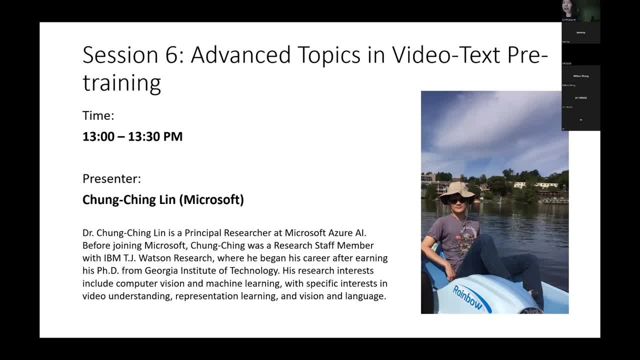 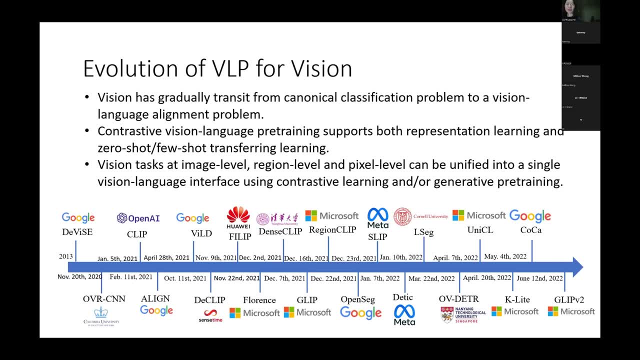 After Chongqing's talk we will have a coffee break in the afternoon. After the coffee break we will start VLP for vision. There has been a surging research interest on how to develop VLP methods to solve the traditional computer vision problems. 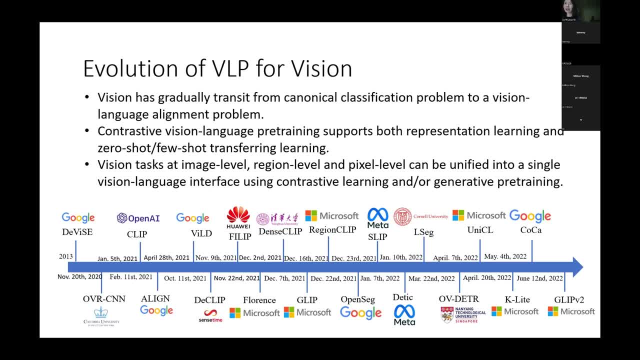 such as classification, object detection and object segmentation. We see that vision has gradually transitioned from canonical classification problems to a vision-led vision. We also see that contrastive vision-language pre-training can support both representation learning and zero-shot, few-shot transfer learning. 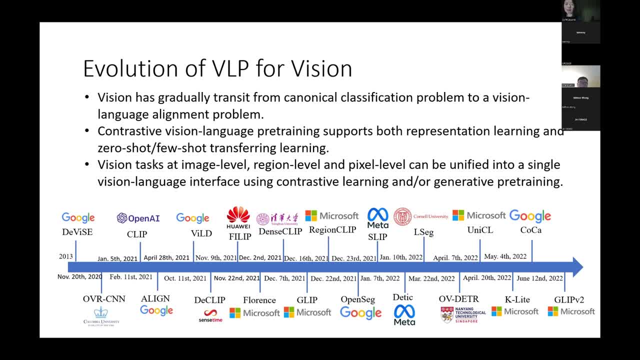 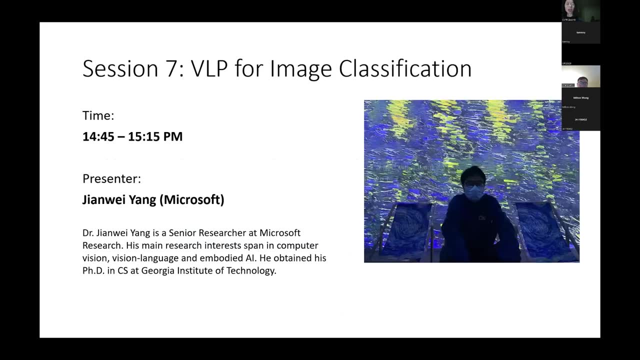 We strongly believe vision tasks at image level, region level and pixel level can be unified into a single vision-language interface using contrastive learning and generative pre-training For the VLP for vision, part Jianwei Yang will first present VLP for image classification. 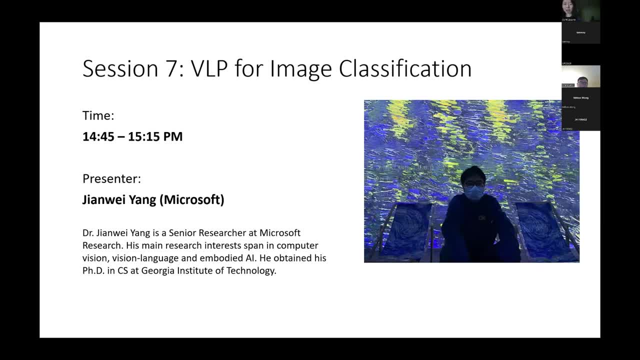 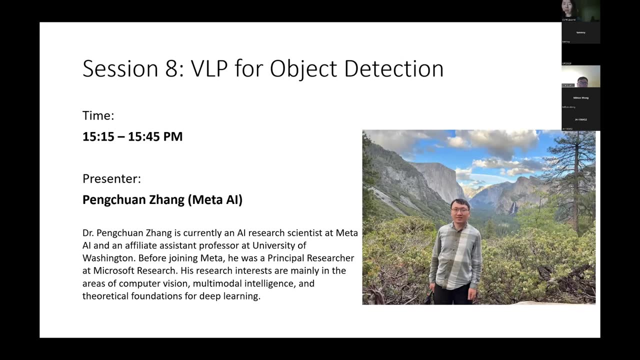 Jianwei is a senior researcher at Microsoft Research. His main research interests span in computer vision, vision language and embodied AI. After Jianwei's talk, Pengchuan Zhang will present VLP for object detection. Pengchuan is currently an AI research scientist at Meta-AI. 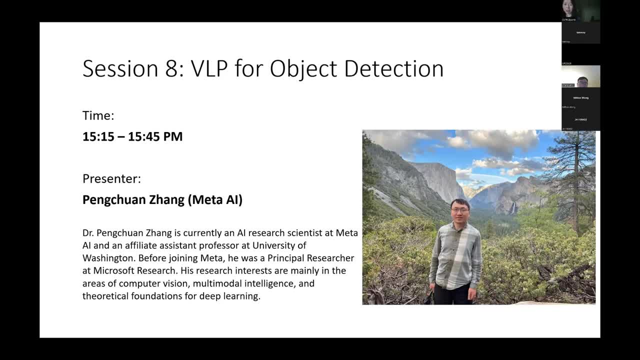 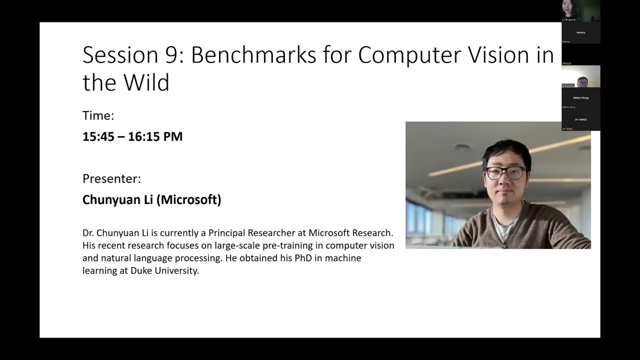 and affiliate assistant professor at the University of Washington. His research interests are mainly in areas of computer vision. multimodal intelligence and theoretical foundations for deep learning will then present the benchmarks for computer vision in the wild. Chunyuan is currently a principal researcher at Microsoft Research. 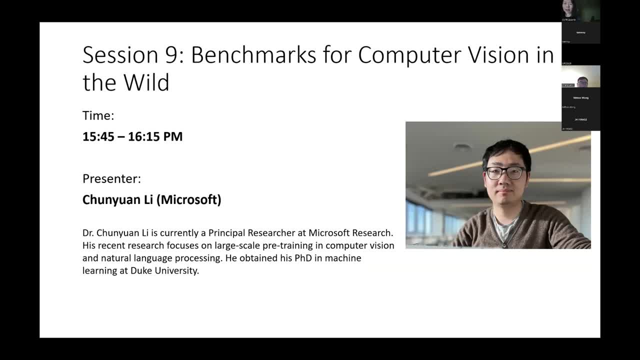 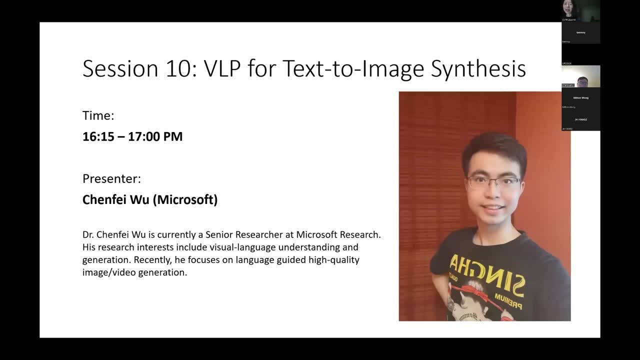 His recent research focuses on large-scale pre-training in computer vision and natural language processing. The last talk of today is presented by Chenfei Wu on VLP for text-to-image synthesis. Chenfei is currently a senior researcher at Microsoft Research. His research interests include vision, language understanding and generation.